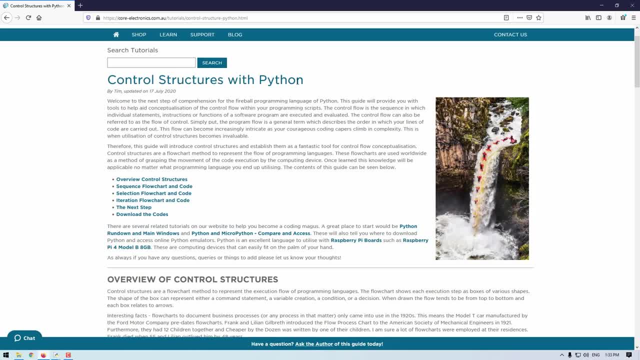 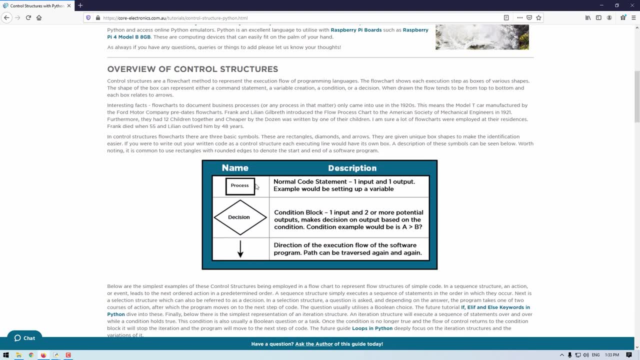 no matter what programming language you end up utilizing, So jumping into the computer. we'll take a look at the online write-up for this guide. So if we scroll down we'll see. these are the different shapes that you'll run into when using control structure flowcharts. 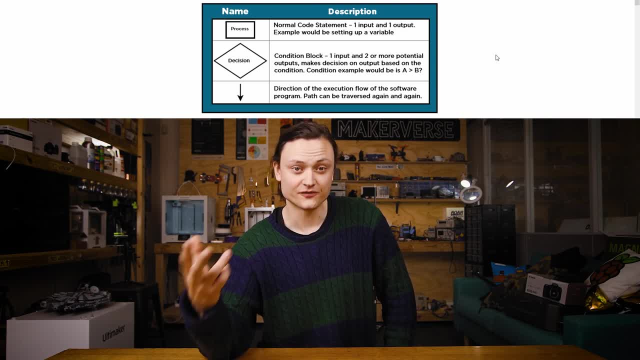 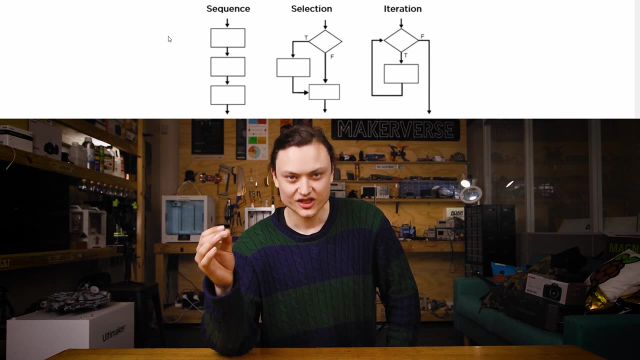 The shape of the box can represent either a command statement, a variable creation, a condition or a decision. When drawn, the flow tends to be from the top to the bottom and each box is related to each other via arrows. So scrolling further down, you can see the simplest examples of these control structures. 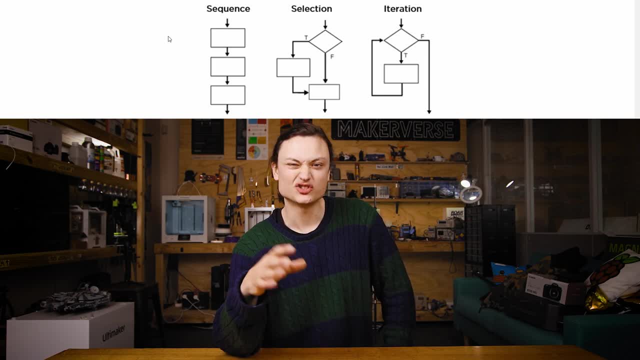 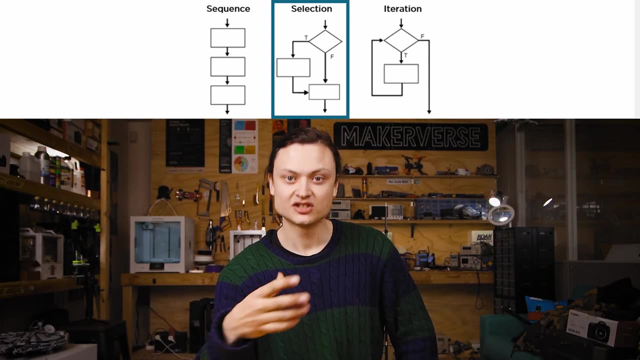 being employed in a flowchart to represent flow structures of very simple code. So, for instance, in a sequence code, an action or event leads to the next, ordered in a predetermined manner. Next is a selection structure. A selection structure can also be referred to as a decision. 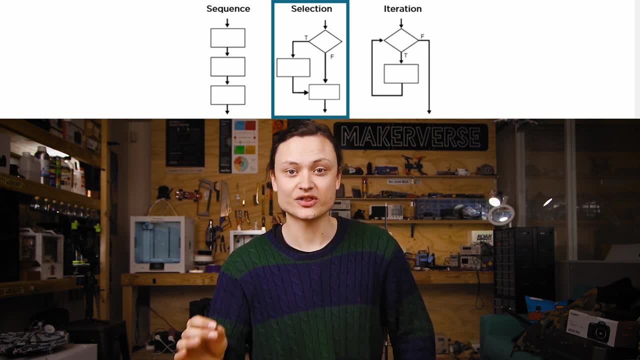 So in a selection structure, a question is asked and, depending on the answer, the program takes one of two courses of action, after which the program moves on to the next step of code. This question is usually a Boolean type. An iteration structure will execute a. 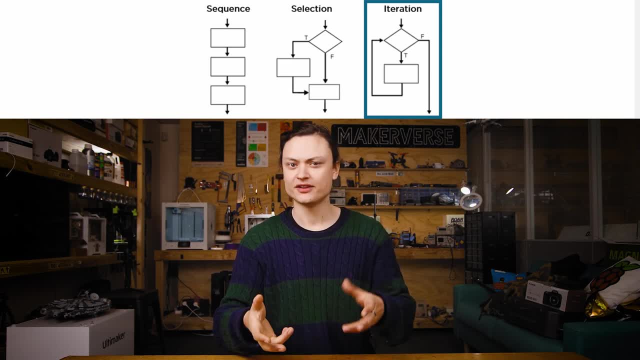 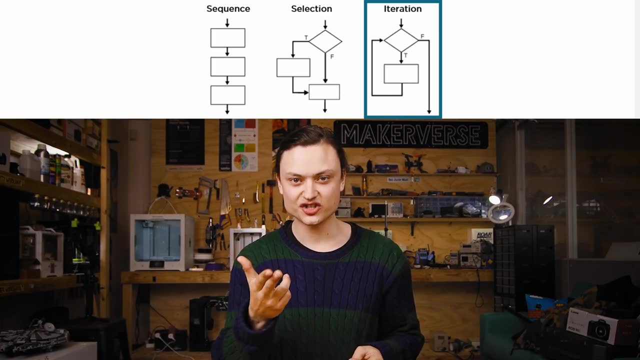 sequence of statements over and over. while a condition holds true, The condition is also usually a Boolean question or a task. Once the condition is no longer true and the flow of control returns to the condition block, it will stop the iteration and the program will move on to the next step of code. 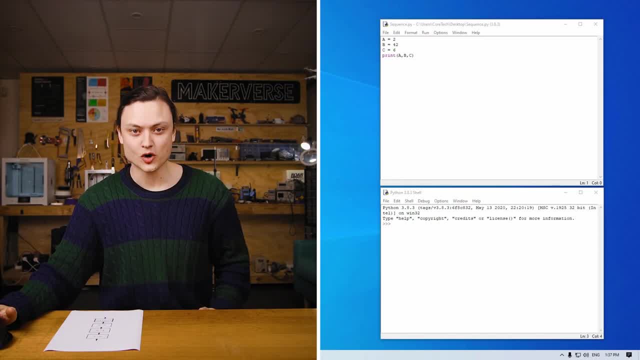 Now on screen. you can see a simple code in the Python programming window setting up several variables and then printing them to the Python IDLE shell. See, when I run this code, it will print A, B and C. You can see the results printed effectively. 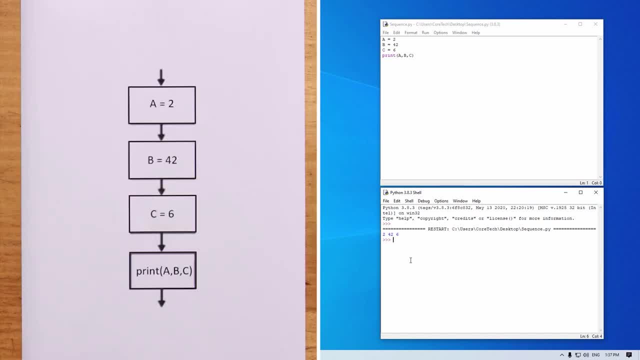 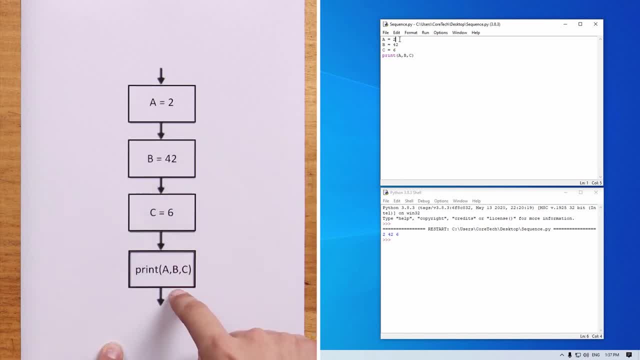 before print A, B and C. so, even though the execution seems instantaneous, it is important to realize a split second, or, more correctly, a split millisecond. This has occurred before this. Now, this is an elegant way to demonstrate precedence. 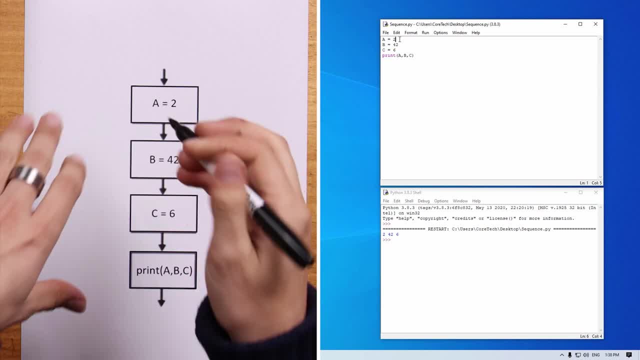 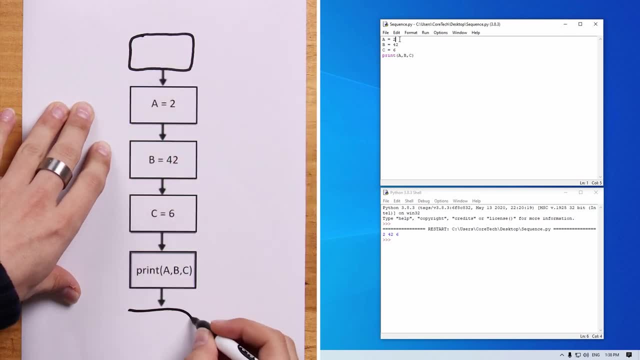 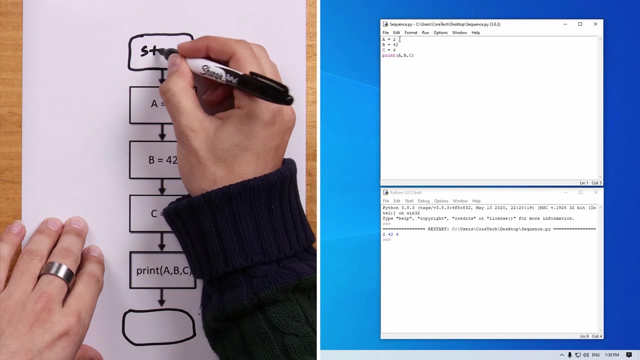 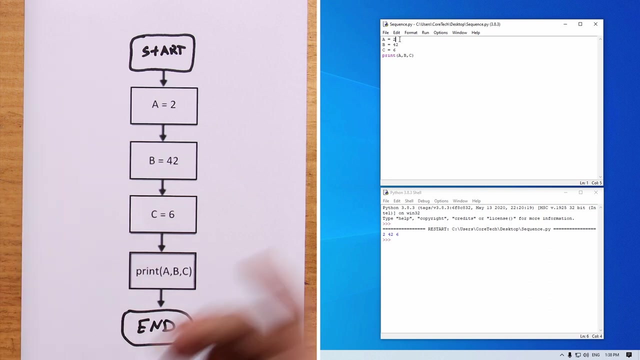 Now worth noting. you may see out in the wild rectangles with rounded corners like so, And these are used to denote the start and end of code And, depending on whether it helped your conceptualization of what's going on in the code, you can use. 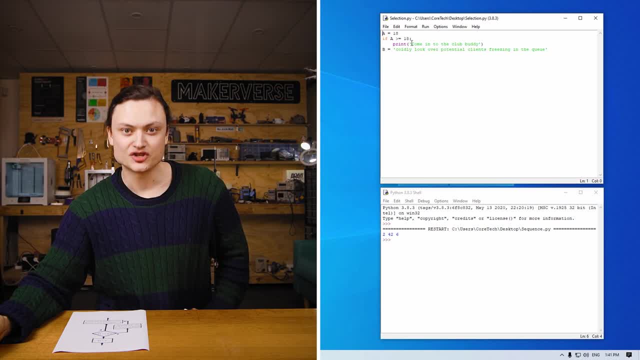 them On screen. you can see a simplification of a bouncer performing his job in Python script form. You have two variables defined and a comparison operator. The first variable, A, represents the client's age and if the client is over 18 years old. 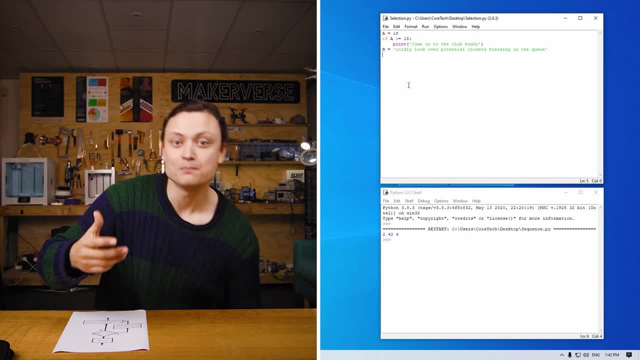 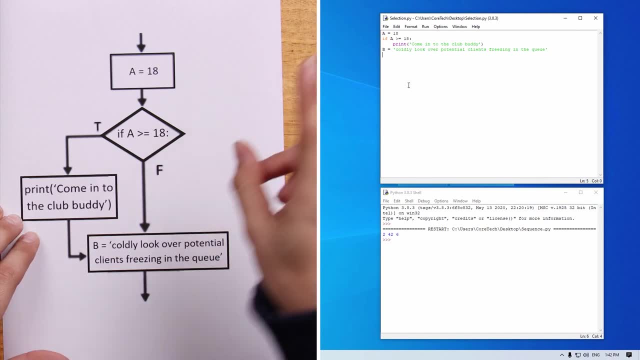 the drinking age within Australia, then they are welcomed into the club. Then B represents the future actions of the bouncer. I have brought to the table a control structure flow chart which clearly demonstrates there are two potential ways for the control flow to get to the stage to produce the variable. 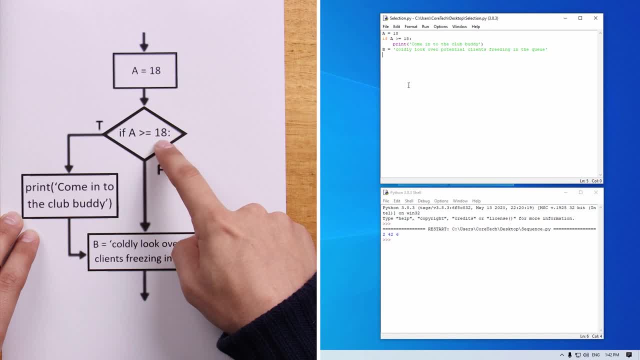 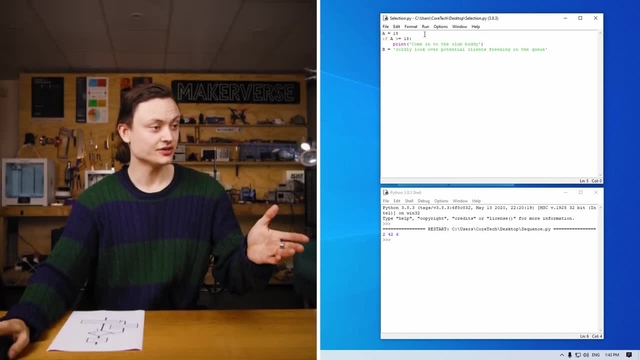 B Down this way: If A greater than equals to 18 is not reached, then it can get this way. If A equals 18 or above, it can go this way. So if I was to run this script right now when A equals 18, you'll see come into the. 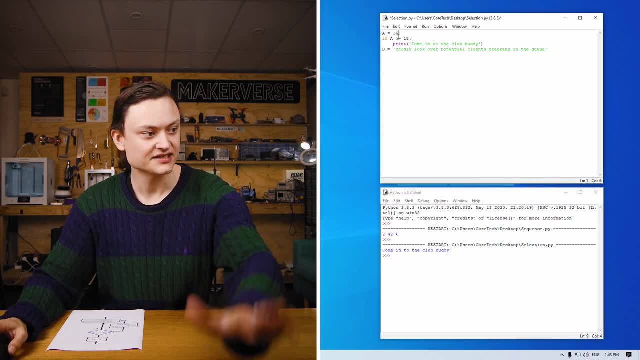 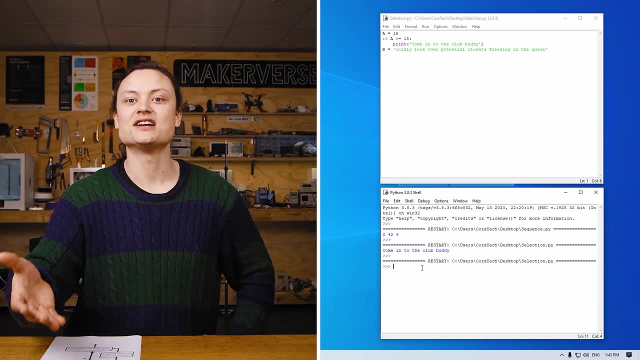 club buddy. However, if this number was less than 18, say 16, run this save. it won't prevent anything. So in this example, if the client is under 18 years old, the bouncer will completely ignore the client. 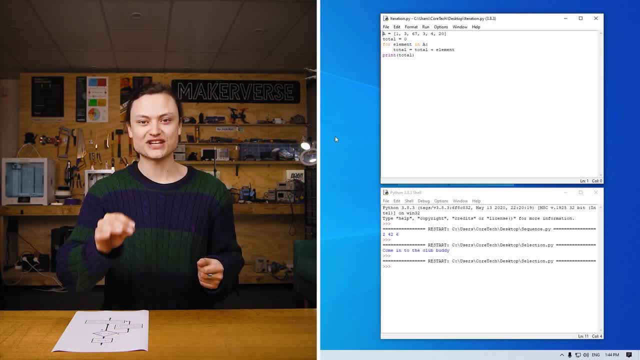 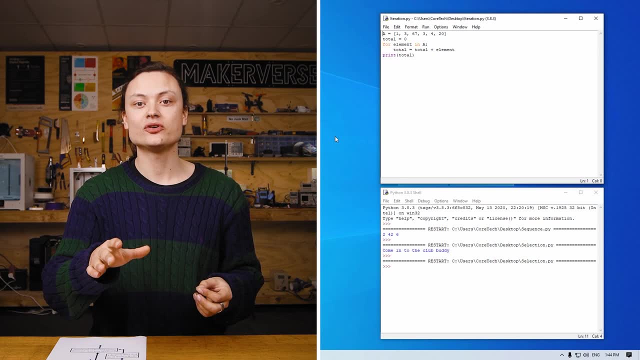 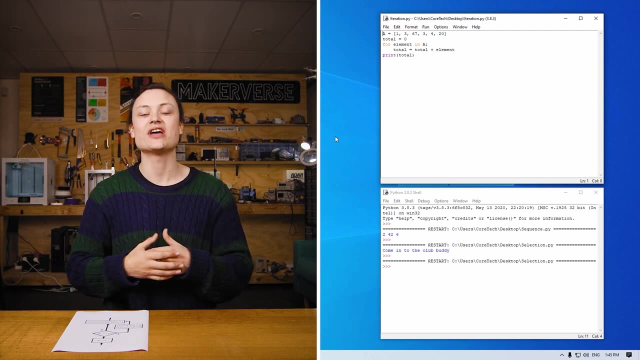 Finally, an iteration structure is one which will execute a set of actions. It will execute a sequence of statements repeatedly. if a condition holds true or a task is incomplete, This specified condition can be thought of as a question or task to the computer. The same question or task is asked again and again until criteria is met or no further. 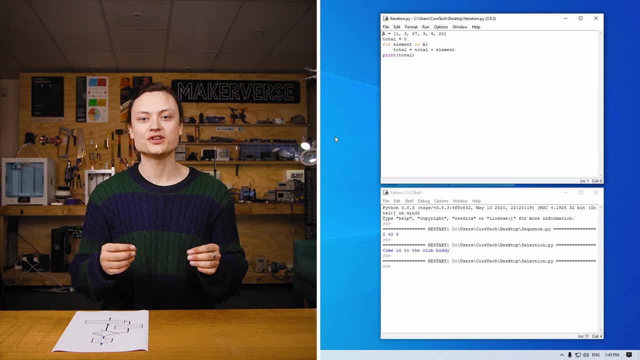 action is required Each time the question is asked or the task occurs. this is referred to as an iteration. Once the condition is no longer true and the flow of control returns back to the condition block, it will stop the iteration And the program will continue to the next step of code.